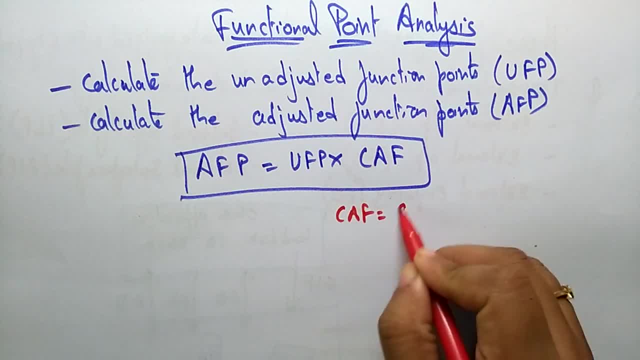 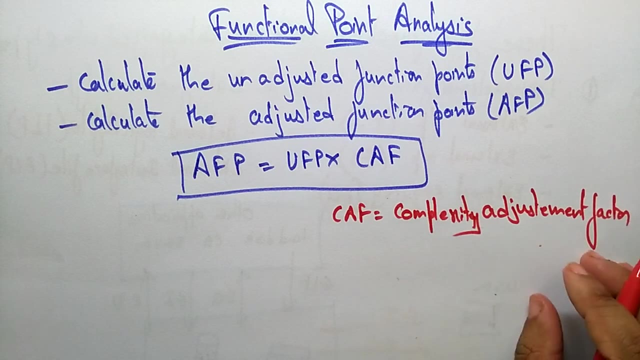 CAF is complex verse. So CAF is complex verse. So this is a complexity adjustment factor. CAF is a complexity adjustment factor. So these are all the terms that are related to theיל, to the calculation of the metrics. if you need to know about the functional point, what are the? 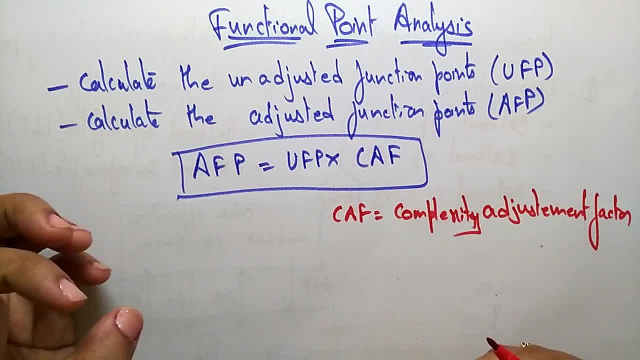 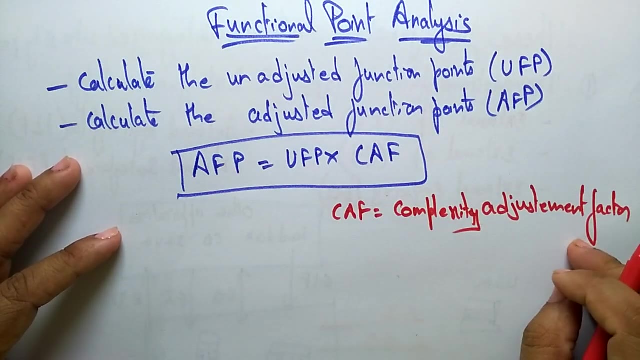 functional points that are functions that are present in the product or the process, and what are the analysis? if you want to know the analysis of that particular standard, particular system, you need to know about the unadjusted function points, adjusted functional point and the complexity adjustment factor. so let me take some simple example of calculating this functional point. 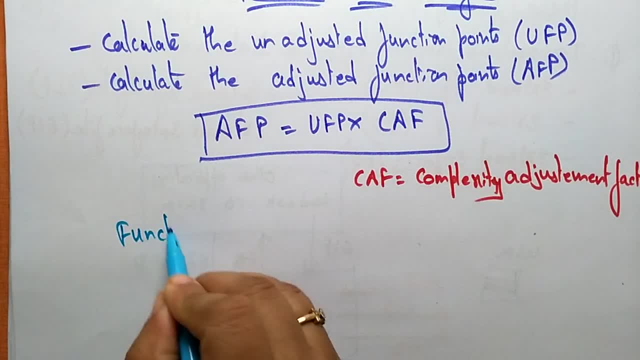 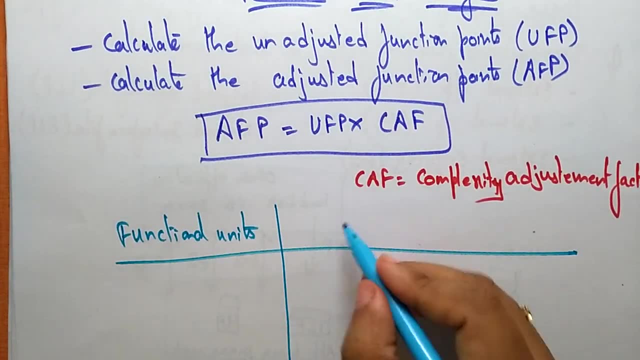 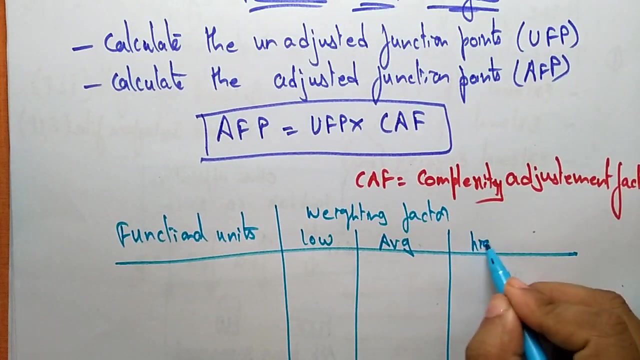 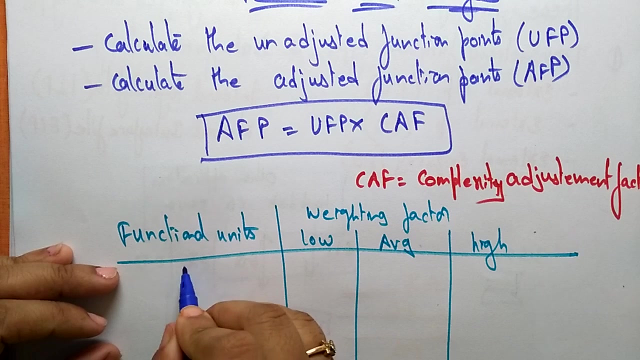 and here i'm drawing one tabular form. these are the functional units and the weight factors, the weighting factors. so the weighting factors are low, average and high. so these are the weighting factors that are related to the functional units. so those functional units may be external input, external output, external inquiries. 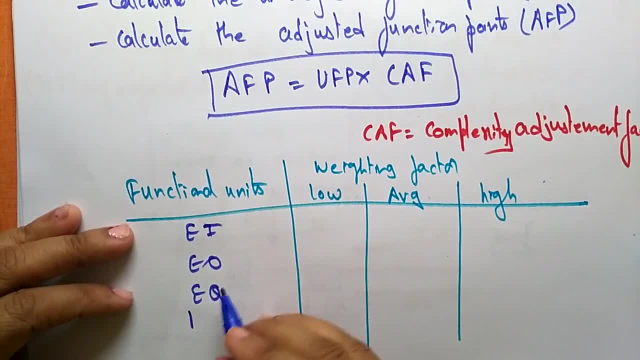 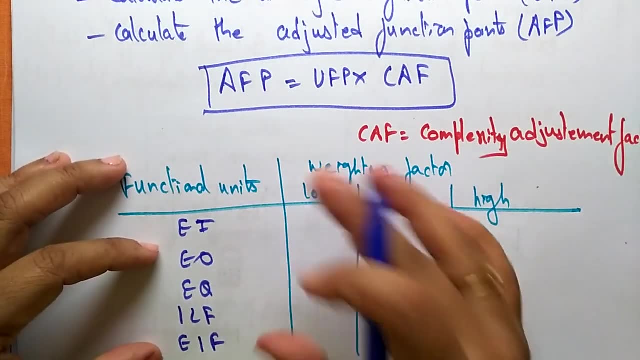 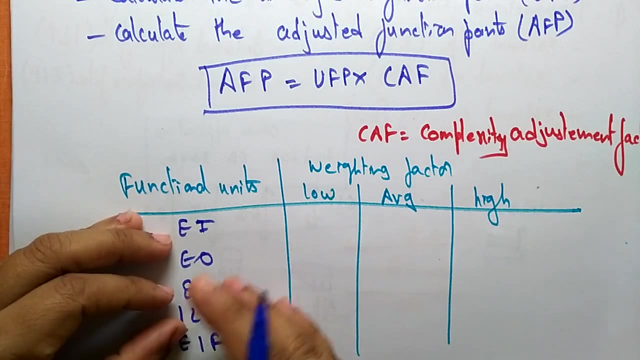 internal logic files and external interface files. so these are totally the five functional units. will be present in any system. so you have to, you need to know, you need to know the functional units. so these are the five functional units, all these five functional units and their weight, weight, weight weighting factors. so the weighting. 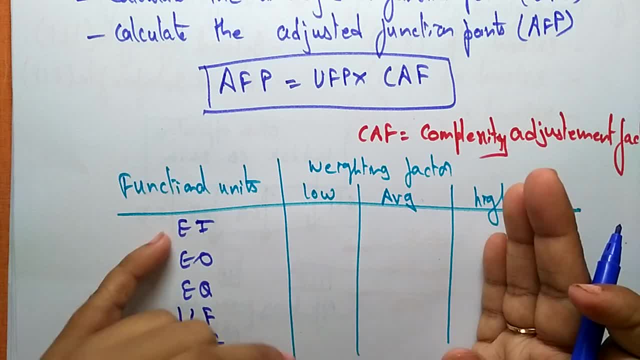 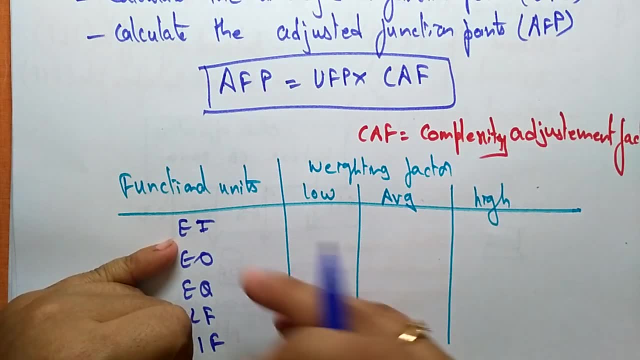 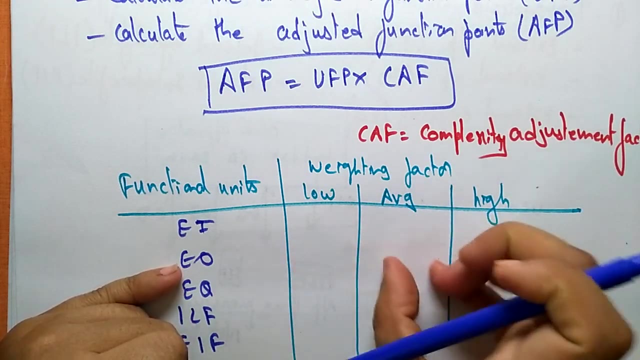 factors is nothing, but the ranks will be according to their complexity. what is the external input input functional unit factor? whether it is uh, it is ranking the complexities with. it is low or average or high. external output is showing the configuration as a low, average or high, like that. 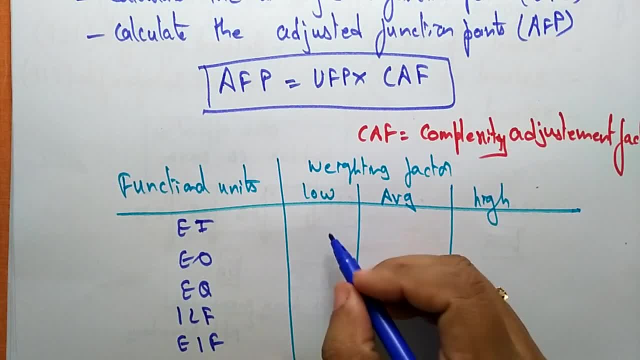 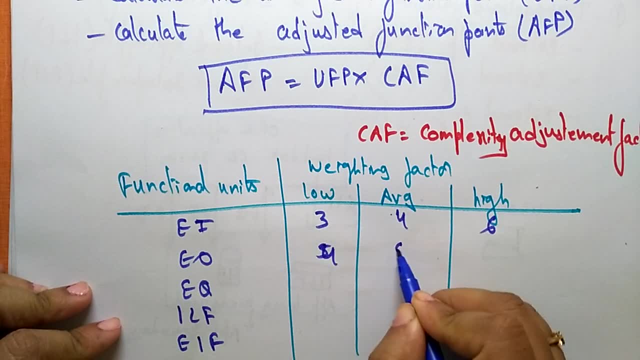 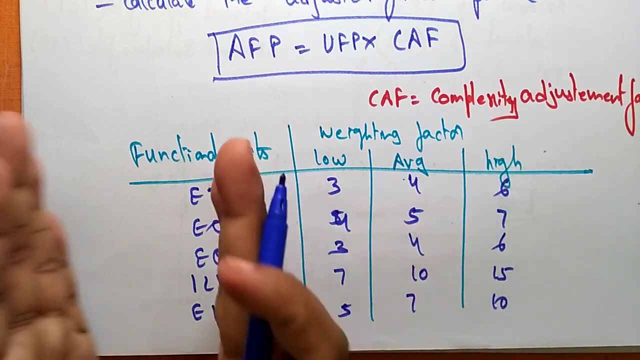 so these are the functional units and those weighting factors. here i'm writing three, four, six. let us take five. oh sorry, four, five, seven, or 3, 4, 6, 7, 10, 5, 7, 10. okay, so this is a tablet from this. five functional units. 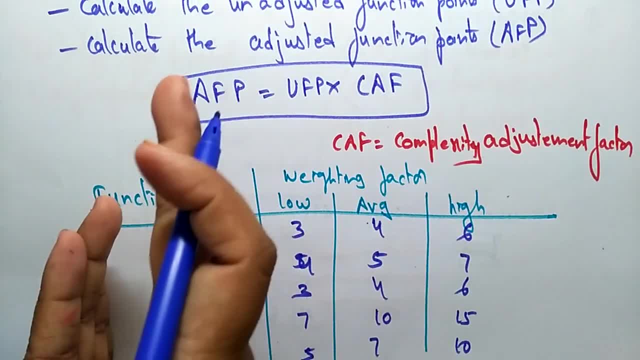 with the help of these five functional units, you are going to actually the fighter functional point analysis that is existed, functional point analysis. okay, so with the help of these five functional units, you are going go ahead and run that documentation to get the functional point analysis. signal loss. 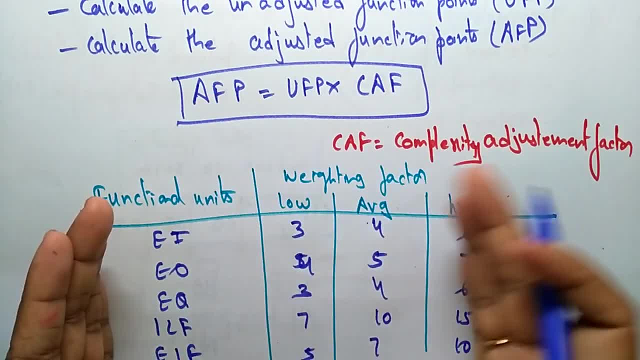 analysis that is existed, functional point analysis. ok, so it also has the same release field. uh uh, functional point analysis that will work on one functionalhrist which this is over the okay, increaseduv customized format in a particular way. um so, with the academic overview of this analysis, that is great to see. 校 ancestor and also a different type of videos. so this is common information for this class, okay, and today we are going to give another time to watch, so suddenly, if you want to know that there are 3 minutes and better words, back to the other Sport tradingcom. 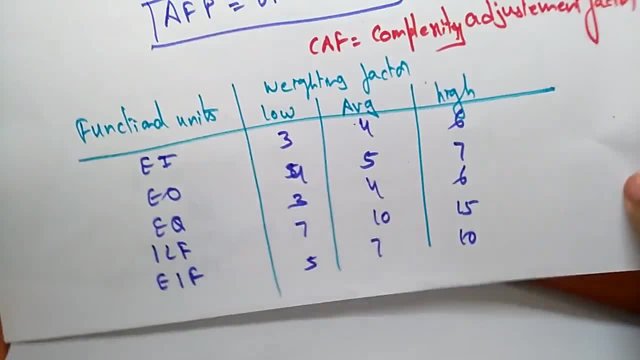 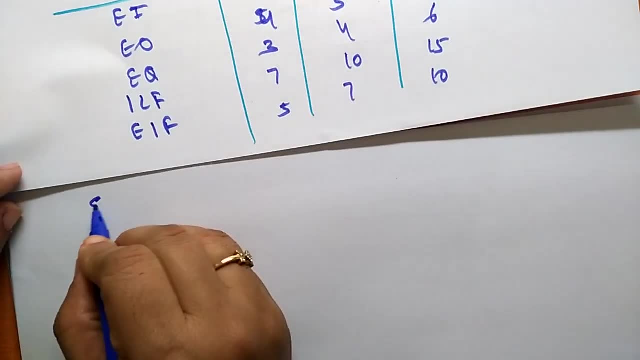 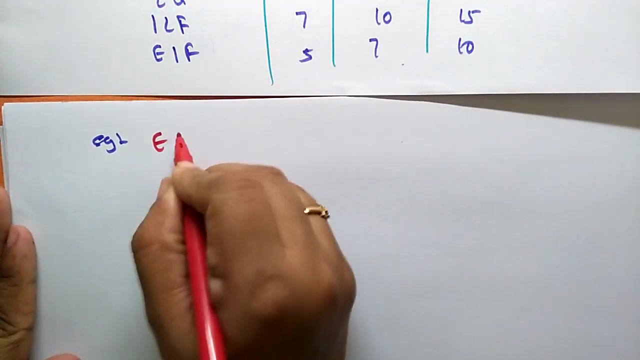 So now let us take a simple example. We are going to recalculate the example by seeing this tablet form. So here I am taking the example. Example was: let us take this EI: EI is equal to 10.. I am giving the low complexity. 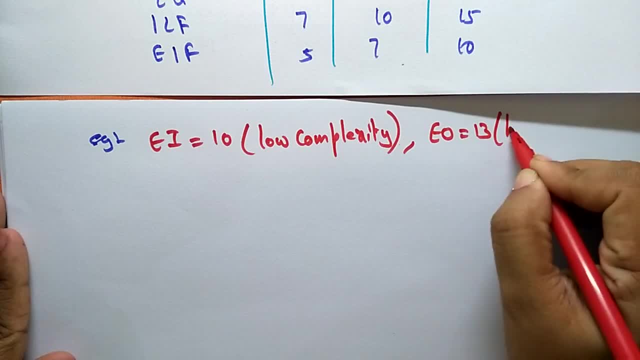 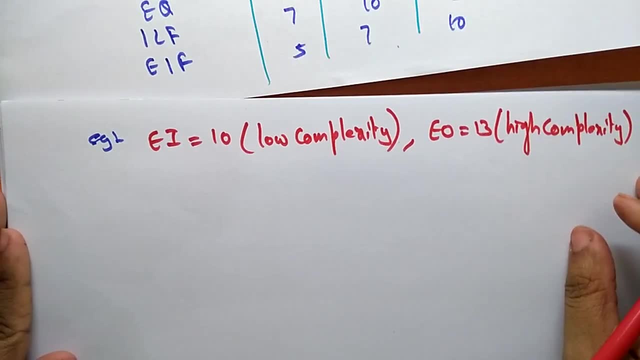 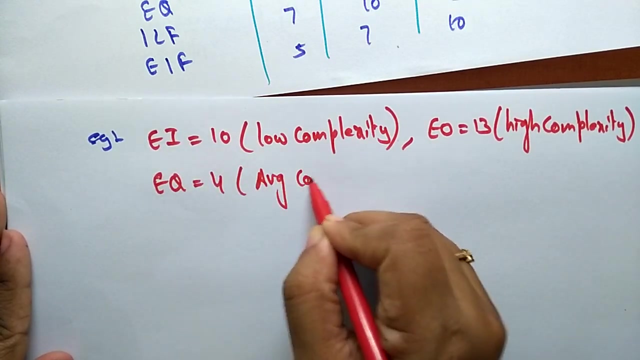 EO external output is 13.. That is a high complexity. The weighing factors- so this is the complexities, the rank complexities And EQ- external enquiries- is a 4. It is an average complexity. The weighing factor is the average. 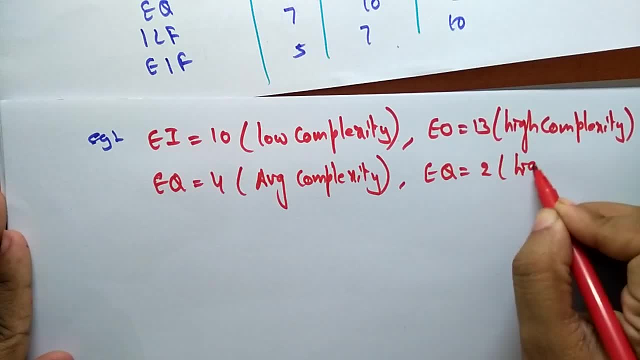 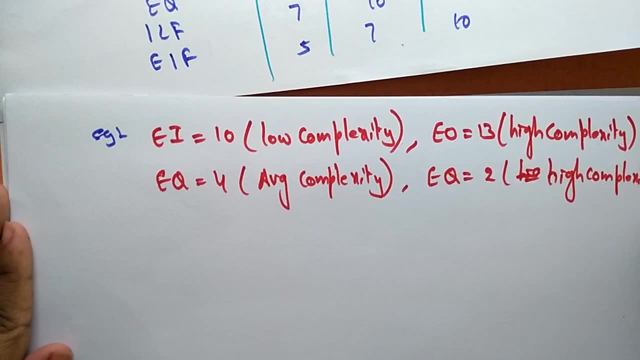 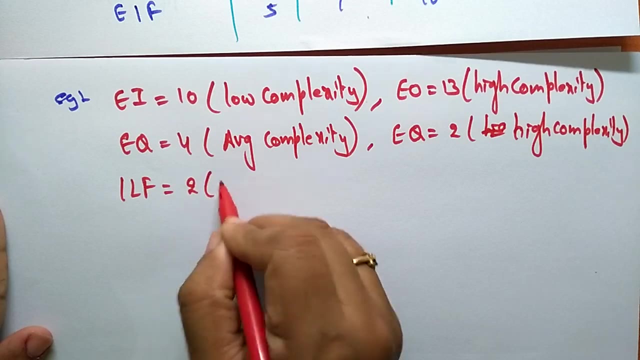 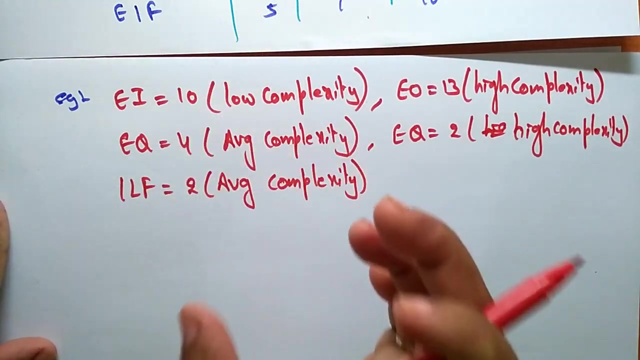 And EQ: 2. Again it is having a high- let us take high- complexity, Okay, And ILF- internal logical files: 2. That acts as an average complexity. So in a system, these functional units are those complexities here I am giving. 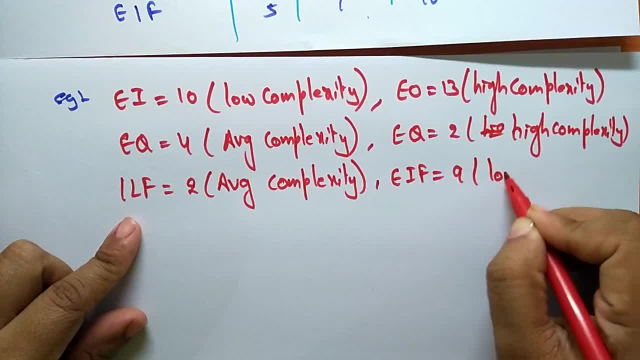 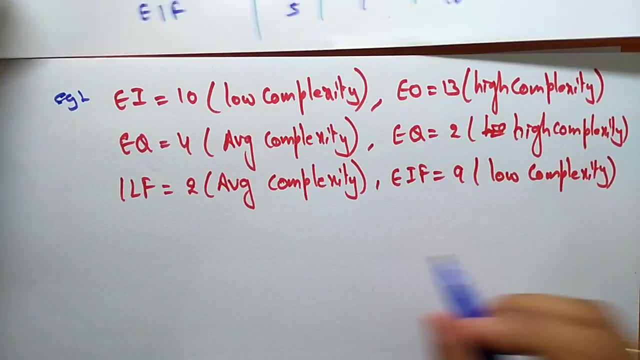 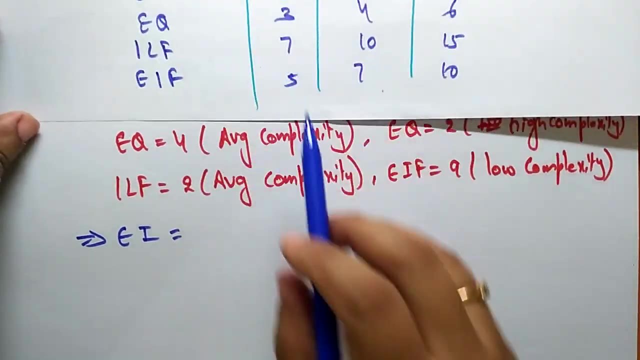 And EIF is equal to 9.. That is a low complexity. Now let us calculate the total complexities of each functional unit. So here, if you want to know the functional unit complexity of ei is, so: they are given 10, they are given. that is a low complexity. 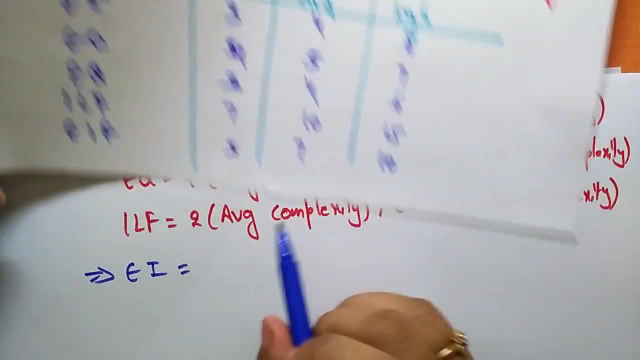 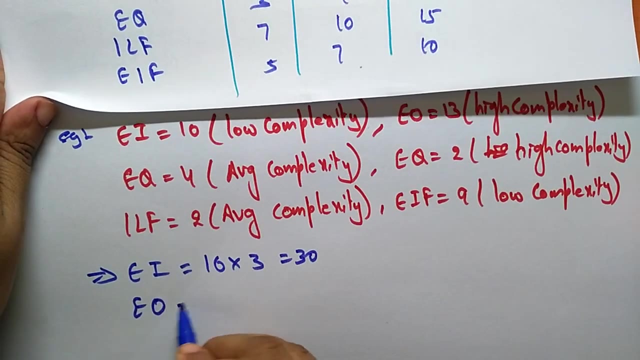 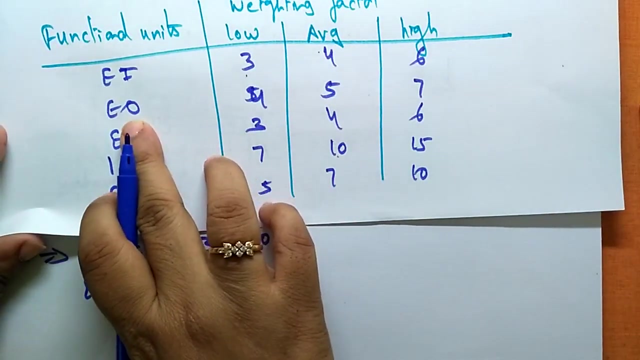 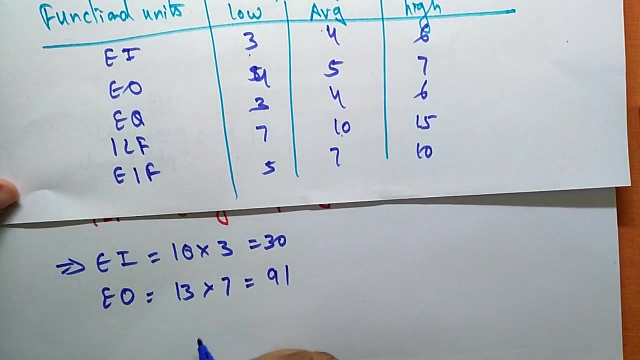 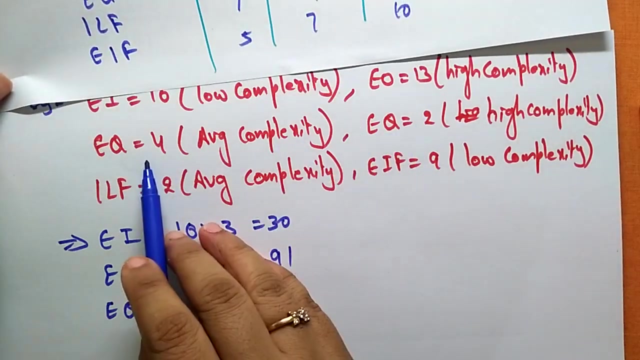 so what is the low complexity here? ei 3, so 10 into 3, 13. next evo, evo 13. they are given and it's showing it is in a high complexity. so what is the high complexity of evo 7? okay, so that is 13 into 7. you'll get 91. next eq, so eq. i'm taking it as a 4, 4 average complexity. so 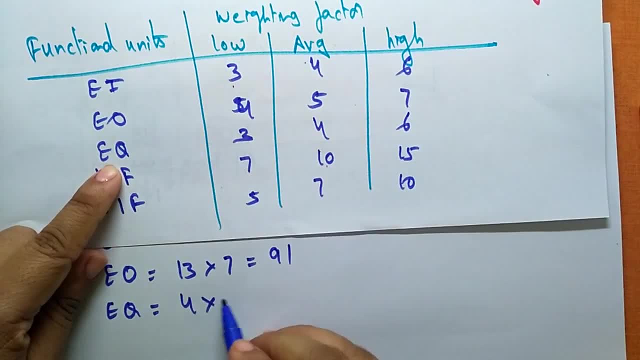 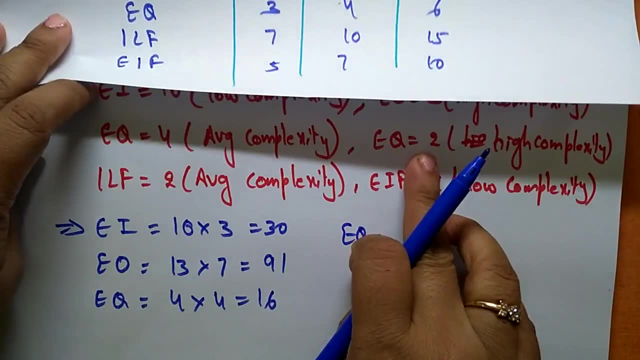 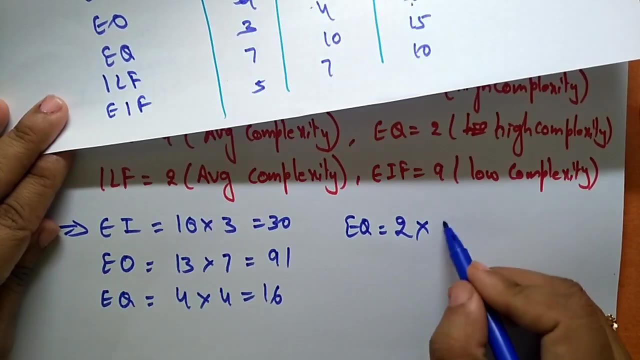 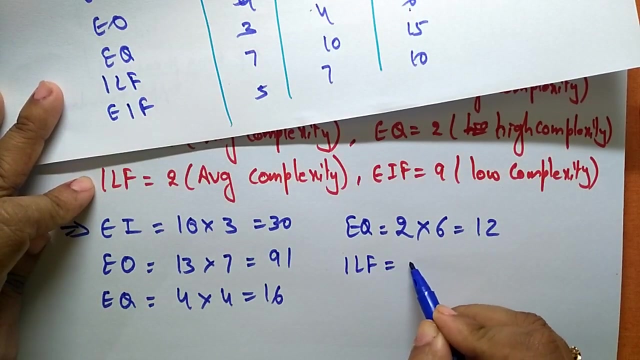 4 into what is the average here, eq average 4. 4 into 4, 16. okay, again i'm calculating eq. eq they are given 2 into high complexity, so 2 into what is the high complexity of eq 6. 2 into 6, 12. next ilf internal logical files. 2 into average complexity. ilf average is: 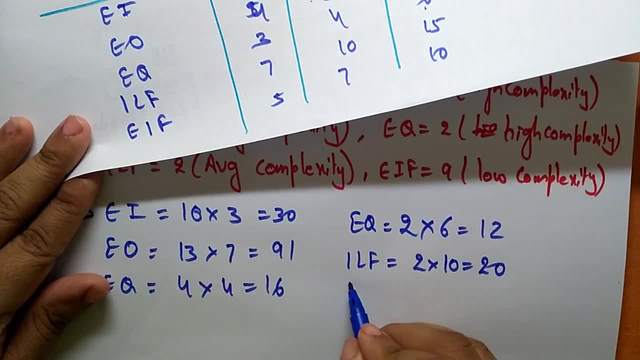 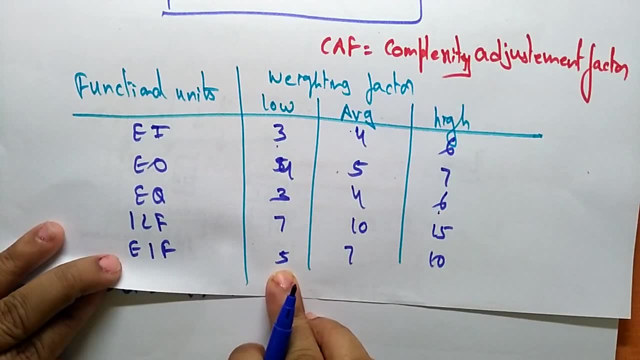 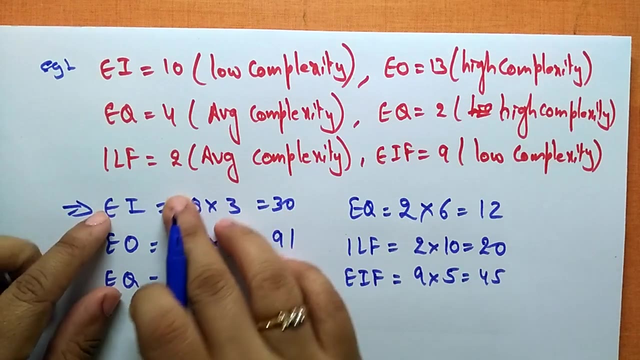 10, 2 into 10, 20. next eif, external interface files: 9 into low complexity. what is the low here? 5. so 9 into 5 will get 45. so just add all these functional units, the weighing factors, according to their complexities. 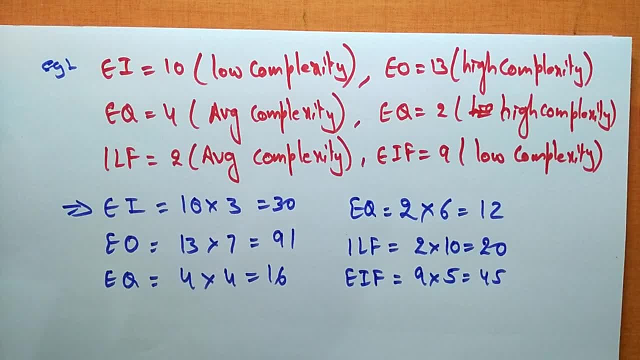 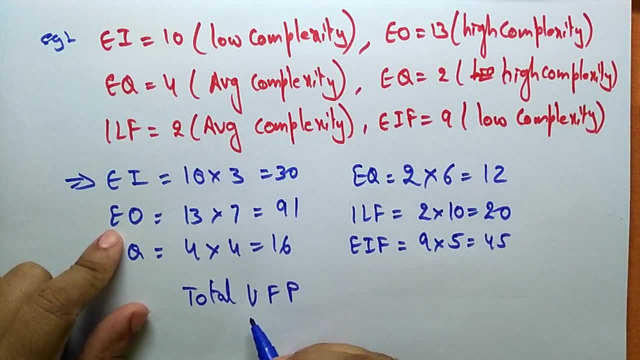 the total. you can say that is here. you can calculate the complex adjustment factor using the. let me write that it is the total. u, f, p means undiff, unadjustable functional point. so these are all unadjustable. now we are calculating the total of the factors according to their complexities. 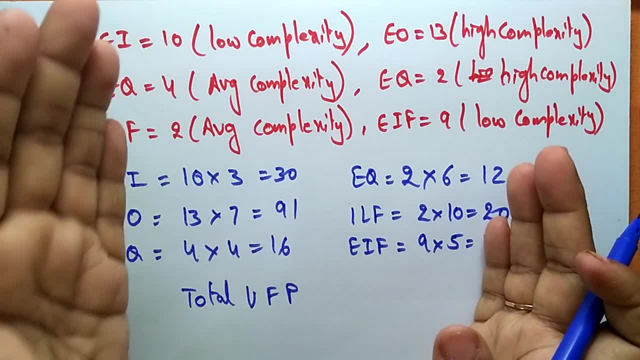 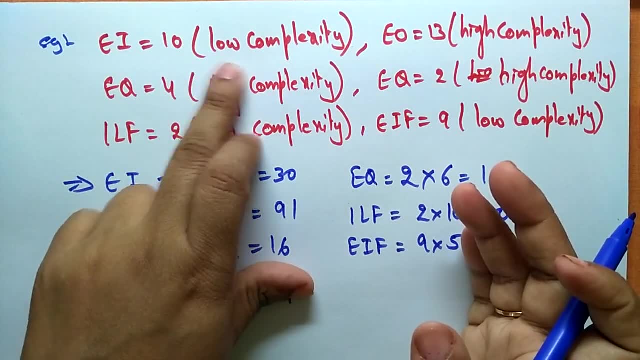 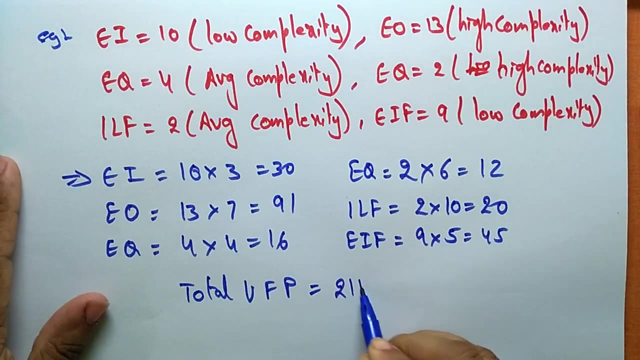 the unadjustable functional points. so the functional points and they are given, and their, their complexities, they are given. so we adjust, multiply those complexity, whatever they are given, and the tabular form consisting of, so you will get the total unadjustable functional point as 214. 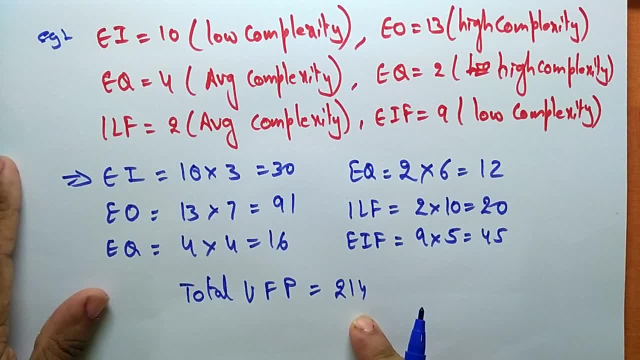 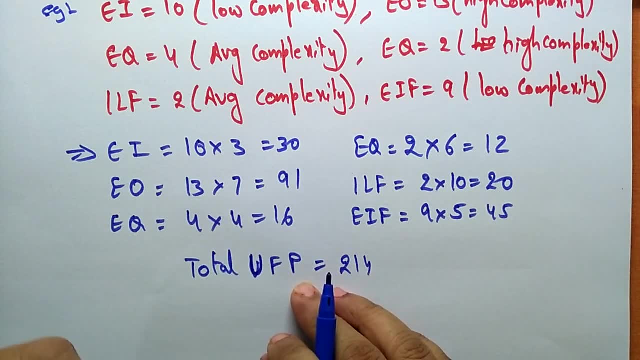 if you are all those things, you will get 214. okay, so 214. now i have to. i i know the unadjustable functional point. if i know, if you want, if i want to calculate the functional point analysis, i need to know the unadjustable functional point into a complexity analysis adjustment factor. so now, 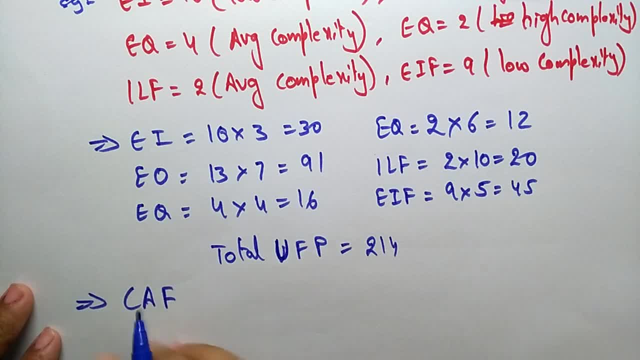 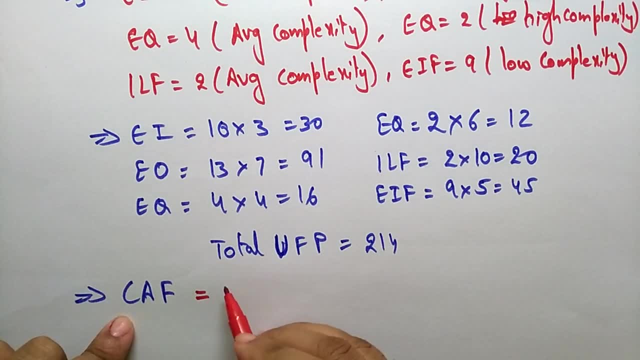 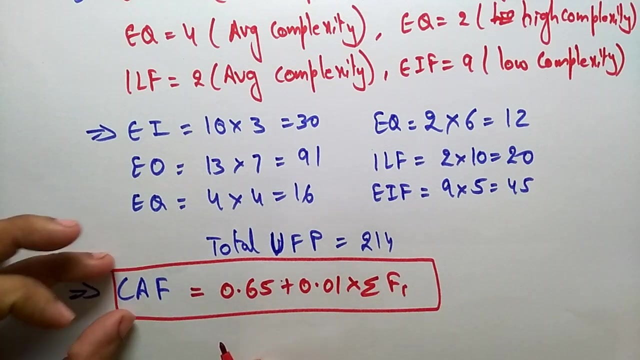 calculate the complexity adjustment factor. so what is this complexity adjustment factor actually? the formula for complexity adjustment factor is equal to 0.65 plus 0.01, equal to 0.65 plus 0.01 into sigma fi. so this is a formula of calculating the complexity adjustment factor. so the standard. 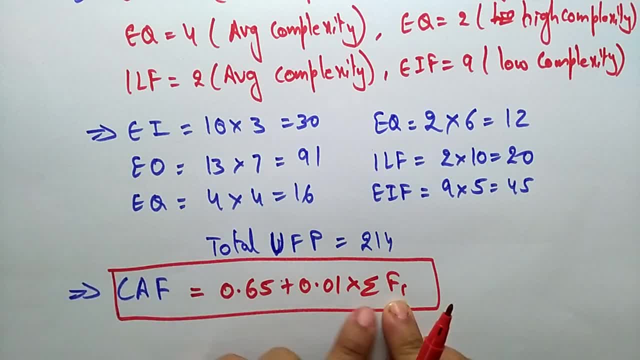 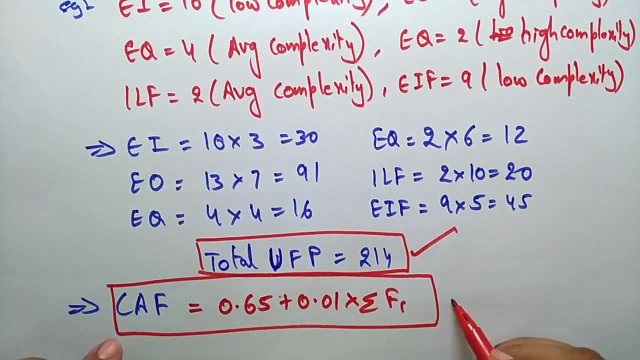 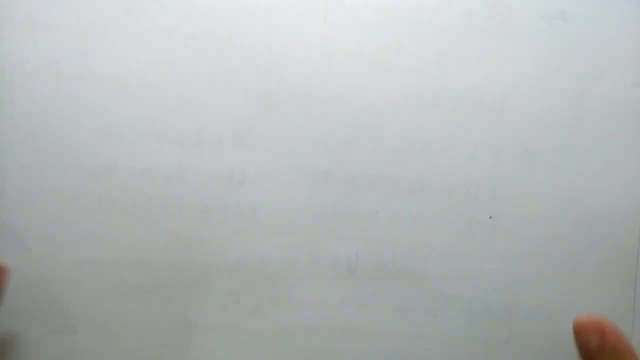 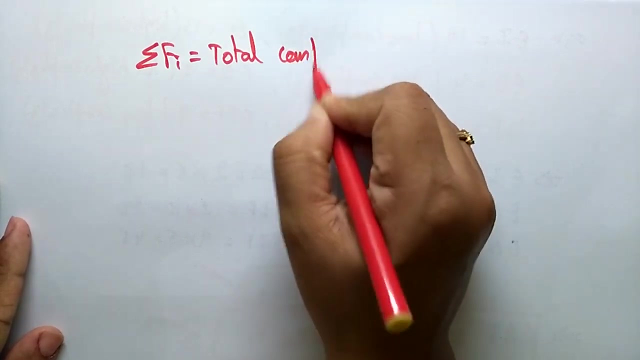 formula. so here i have to know about the sigma fi. what is the sigma fi here? so total ufp i calculated, now i have to calculate it cf. cf means i need to know sigma fi, how i am going to calculate the. so, first of all, what is sigma fi? sigma fi is nothing but total complexity, adjustment value. 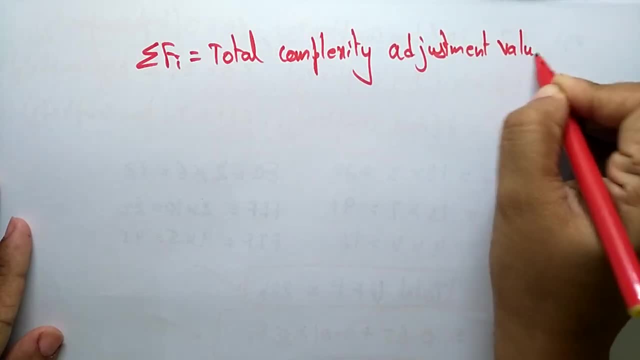 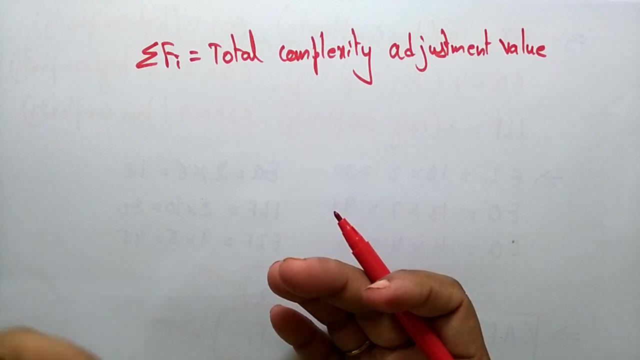 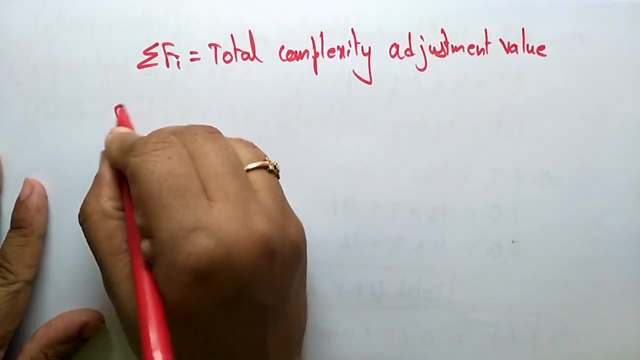 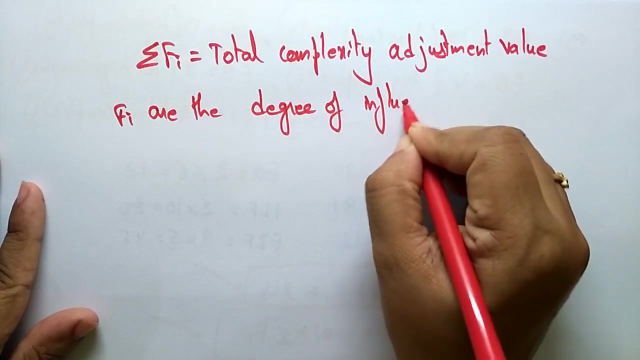 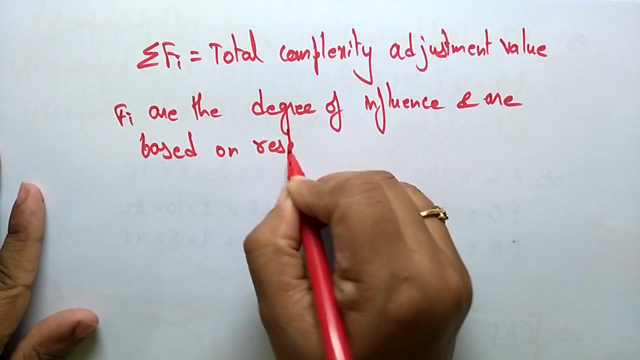 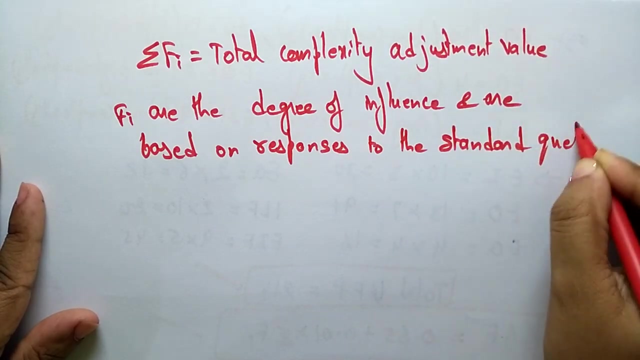 so how i will get this total complexity adjustment value? on which basis? on what basis i can get this total complexity adjustment value actually here? the fi is nothing but here. fi or the degree of influence and or based on based on responses to the standard questions, to the standard questions. so fi is just a degree of influence or based on response to the standard. 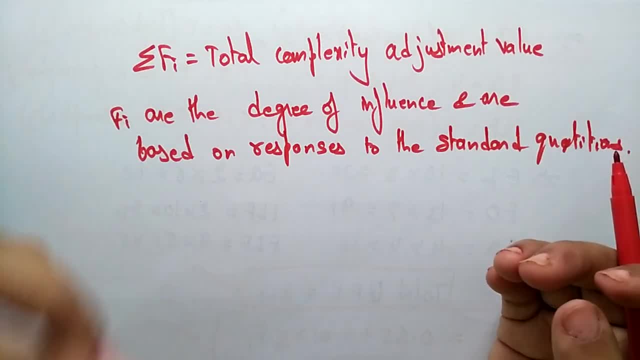 questions. so, whatever the questions they are asked to the standard questions so i can get this total complexity adjustment value on which basis i am asking. okay, if the user wants to calculate the system functional point, functional point analysis, they need to know the degree of influence or they need to know what are the questions. they 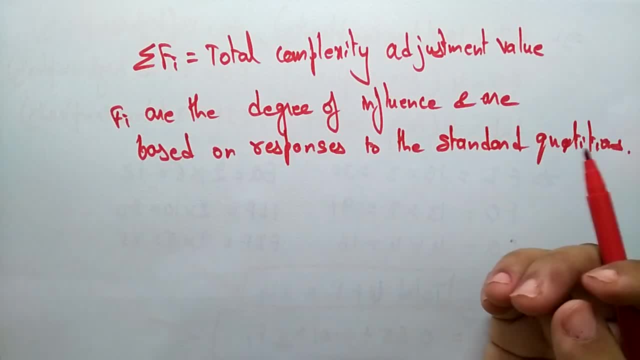 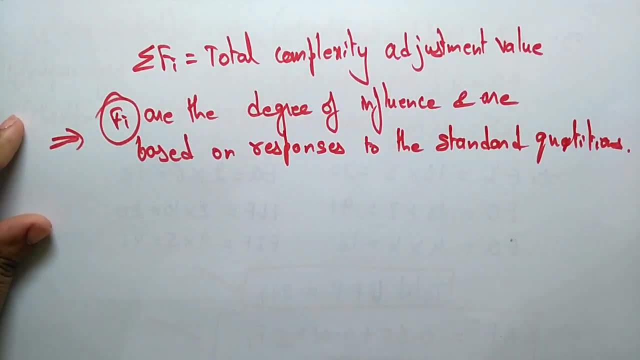 are asking: and what is the degree of that question? so let me explain that. now i am going to explain how i am going to calculate the fi. so how can i find the degree of influence on the standard questions? okay, so actually, rate of each factor can be scaled. 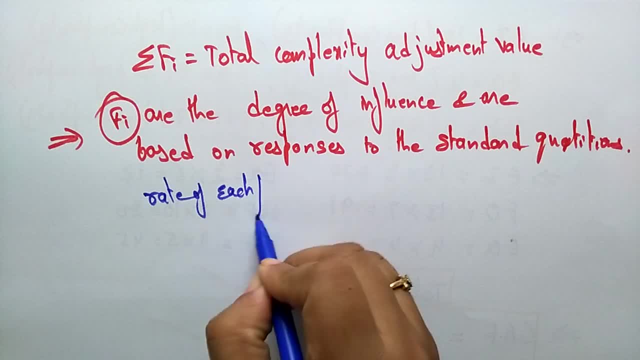 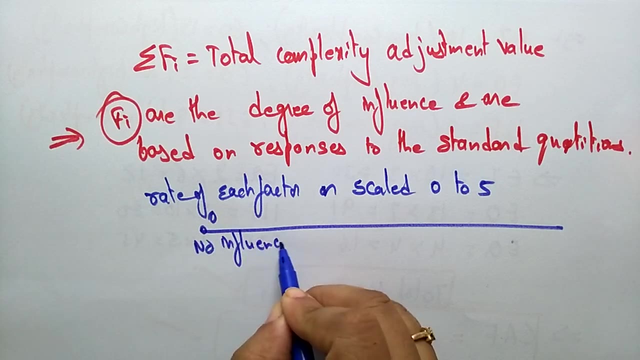 rate of each factor that is a functional element factor can be scaled on. scaled zero to five, the rating will be from zero to five. zero means no influence findings. it is a essential, it is very important. and one is incidental, two is incidental and five is by incidental. two is by incidental. so if one is by incidental and one is incidental, 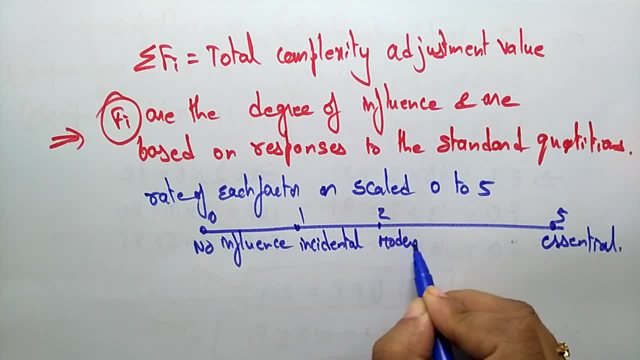 then phones arrest if one is incidental. can the variable class is resolve and function of each object with every county or country by scenarios with everyone may disagree with thatbn. sorry, please work for a moment. if you think about to the question part now, wait a minute. is moderate, 3 is average, 4 is significant, so this is a scale range. 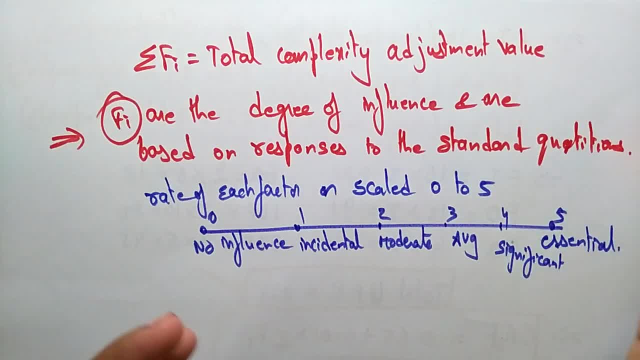 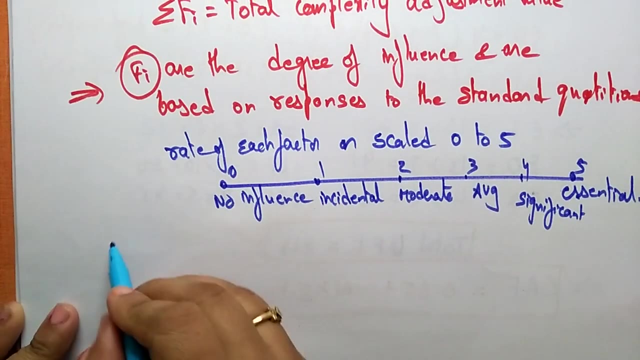 means, if you want to know that, that standard question range, the scale will be from 0 to 5. okay, if that question is standard to your system, that that is a degree of influence. so let let let me take in this example I am considering some standard functions, the number of factors considering here or so in my 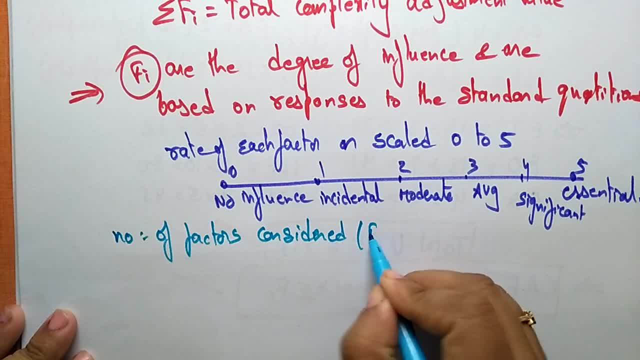 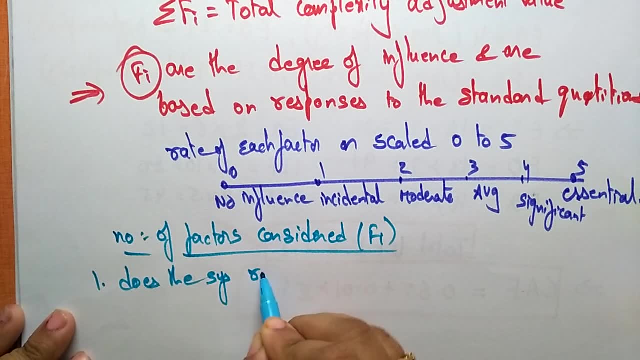 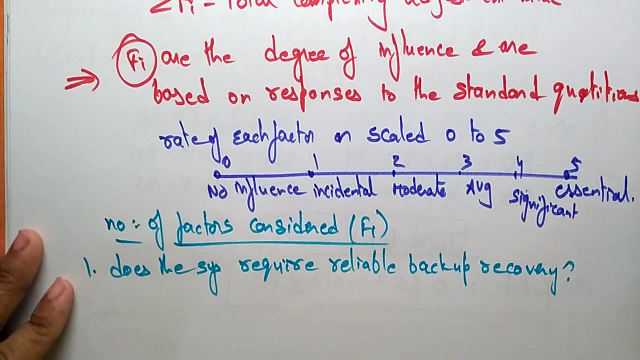 system. I am going to consider some standard number of factors, that is, fi or so. let us take the first one: does the system require real able backup recovery? so then, the first factor I am considering in my system means I want to know the calculation, that is a. does the system 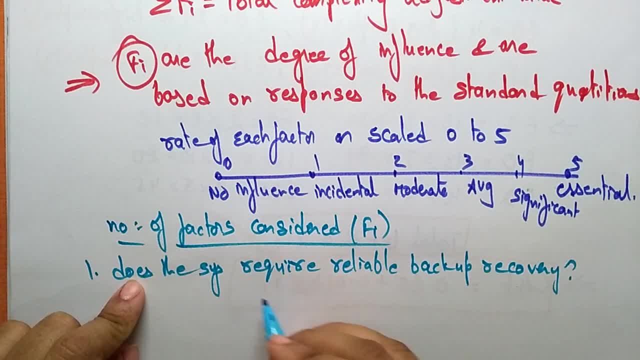 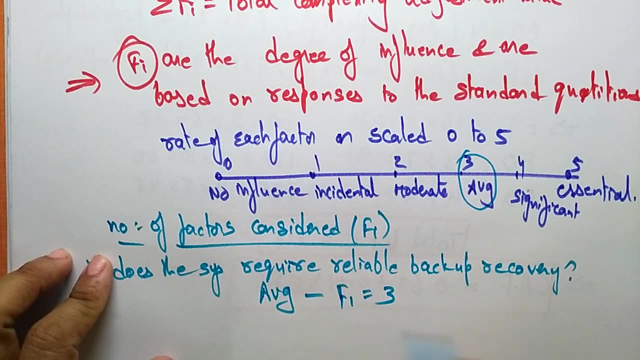 requires real able backup recovery. is there or not? suppose if it is yes, so if it is this, the answer is the suppose I am saying it is average, the system backup is average means. average means 3, so you call it as f1 is equal to 3 means. 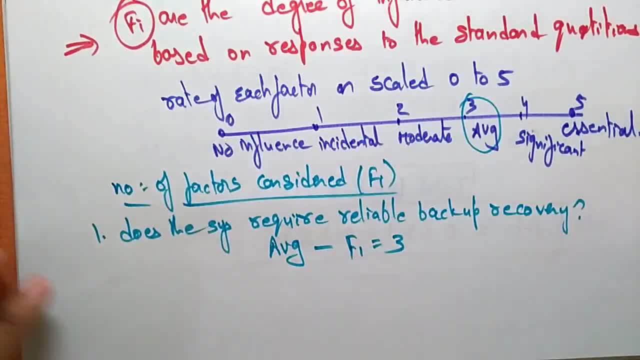 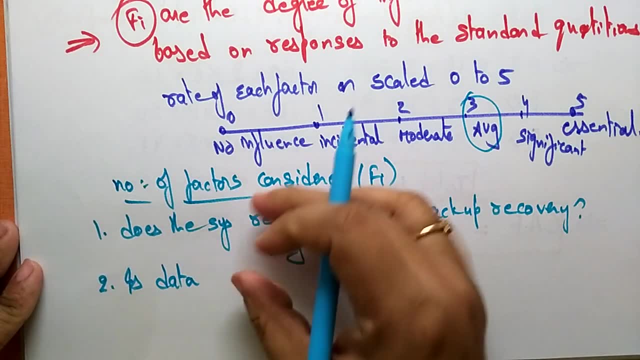 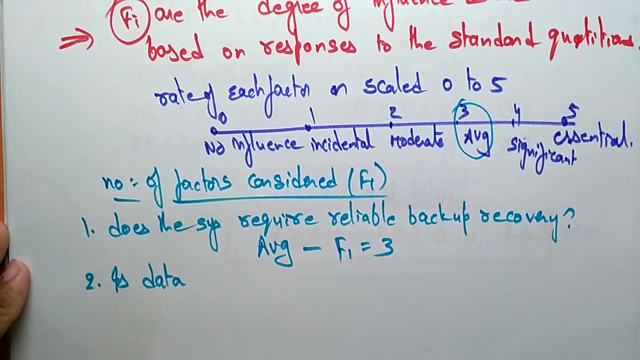 the first factor, that is, f1, is 3. in the same way, second is data communication. so it's everything. the F is based on the number of factors that are considering while you are going to be calculate on system means the number of factors that we are considering in the system. so here I want to know these data communication. 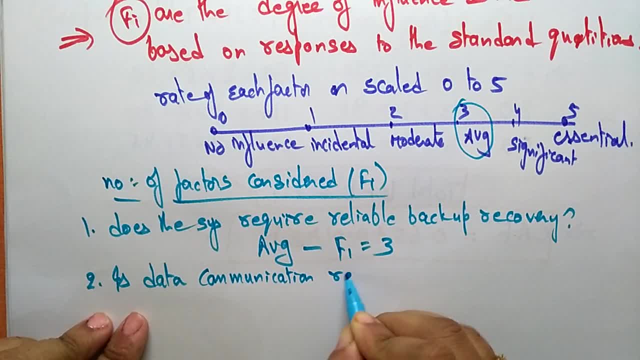 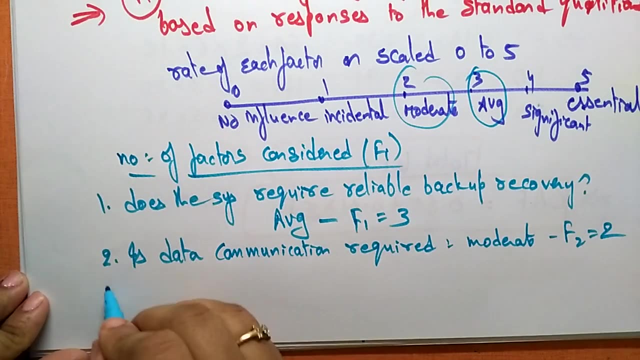 is communication required or not. so I am saying, okay, if my system, the data communication required, may be a moderate. moderate means 2, that is, f2 is equal to 0.5.. equal to 2. so in the same way, 3- i'm is distributing processing- is available or not. 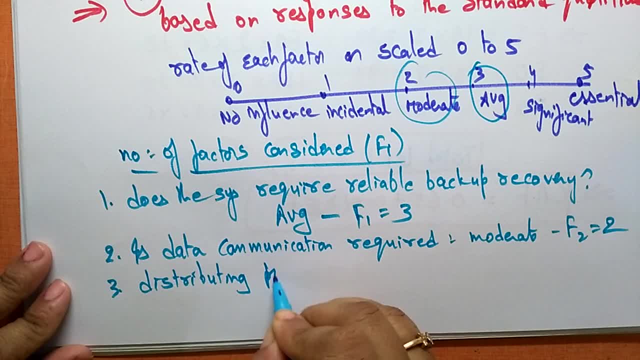 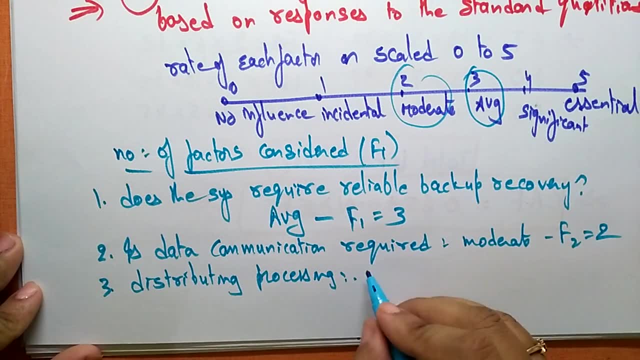 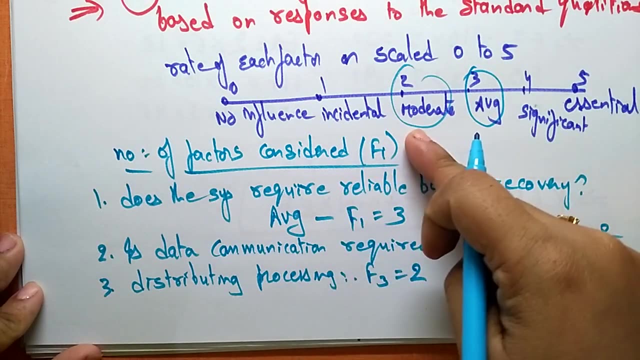 distributing processing is there or not? okay, i'm taking it is as a okay average. averagely, the distributing processing will be performed. means f3 is equal to 2. that is average is sorry. average is i'm taking moderate. let us take moderate. it is 2 and the fourth: 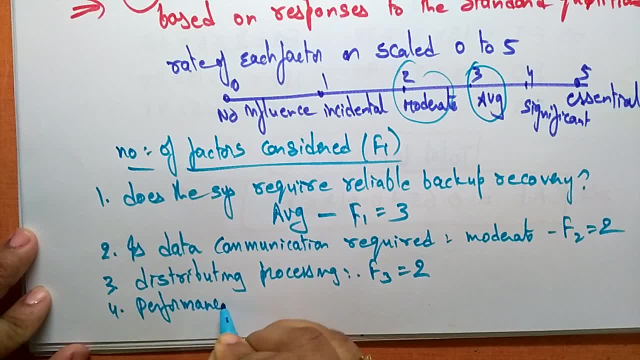 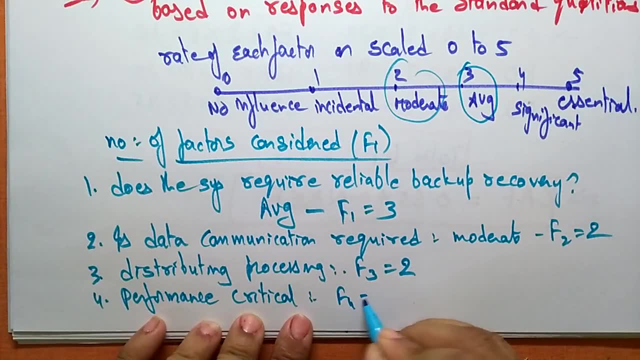 question is: performance critical is how is the performance critical in the system? so i'm taking f4 is equal to, let us take it is, i'm saying it is essential, the performance critical. i have to take it as an essential point. so the scale is f4 is 5. uh, in the same way i'm taking 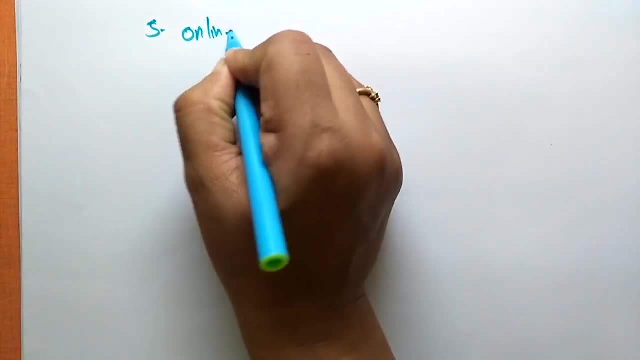 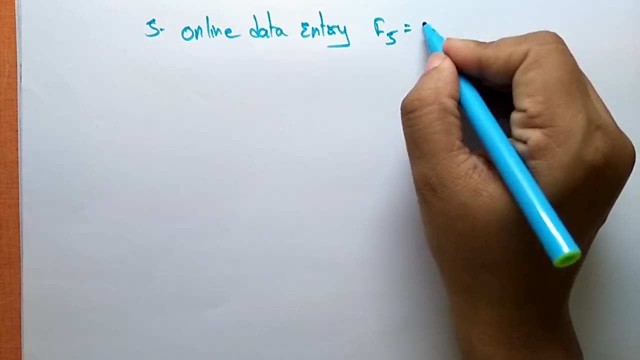 is fifth one. online data entry is available or not. so i'm taking dot. online data entry will be 那我們 there. in my system f i z should be average. average means 3, so then you just calculate all: 5, 1, 2, 3. 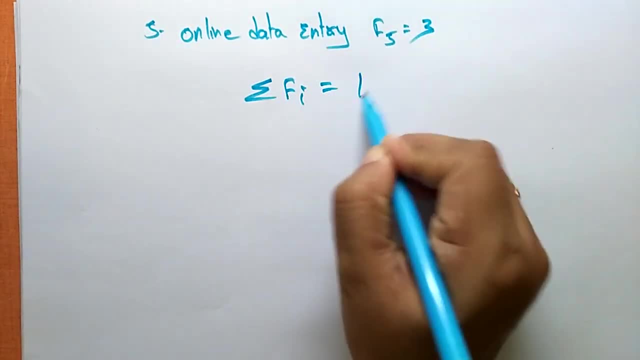 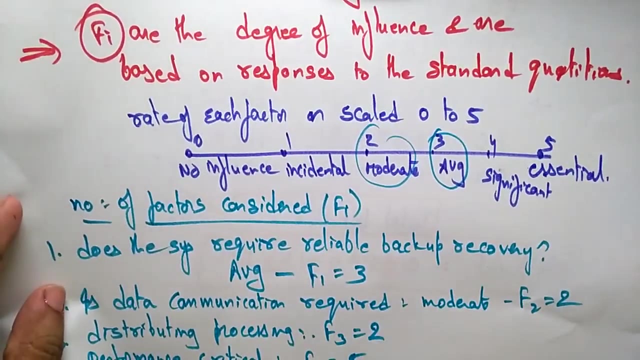 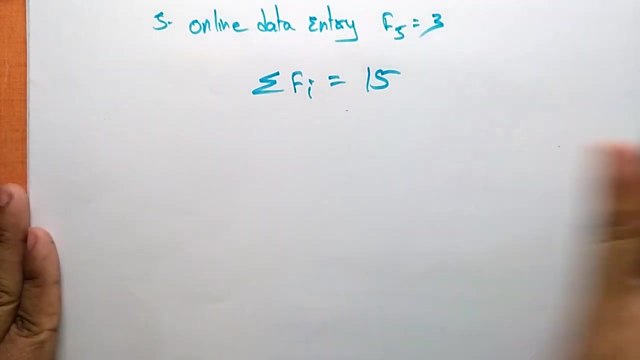 4, 5. add: that is sigma f i is equal to, you will get total 15. how i will get the 15? okay, just i am adding: f 1, 3 plus 2 plus 2 plus 5 plus 3, you will get sigma f i is equal to 15. so now now calculate. 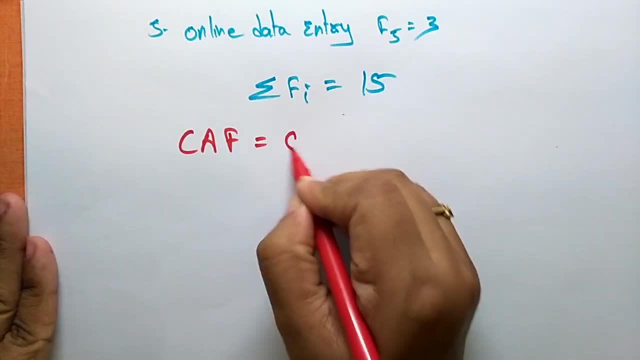 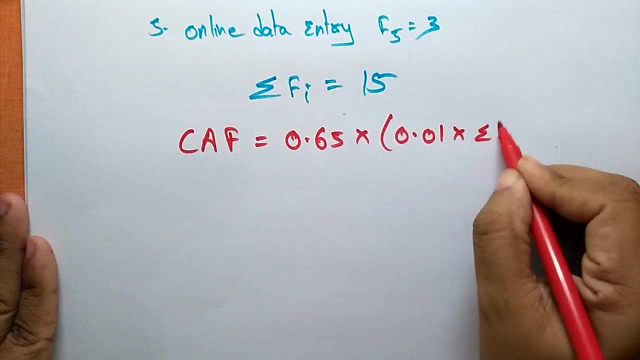 the cf. cf is equal to 0.65 into 0.01 into sigma f i. actually the formula is: sigma f i 0.65 into 0.01 into f. i means 15 here only. i considered only the five questions. number of factors i. 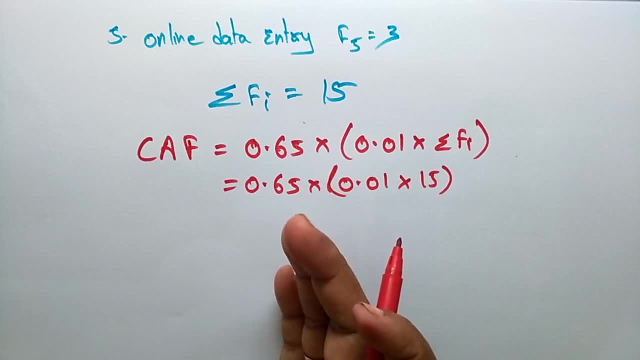 considered in my example is only the five factors, so the. if the number of factors are increased, the system uh, the system uh, this f i will be increased means the calc will be more. so i'll get around 0.8. so i know the uaf ufp. 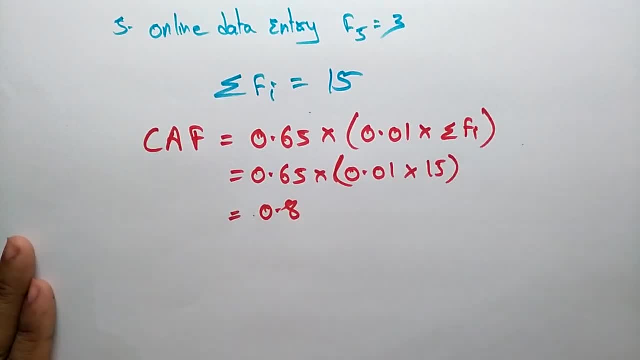 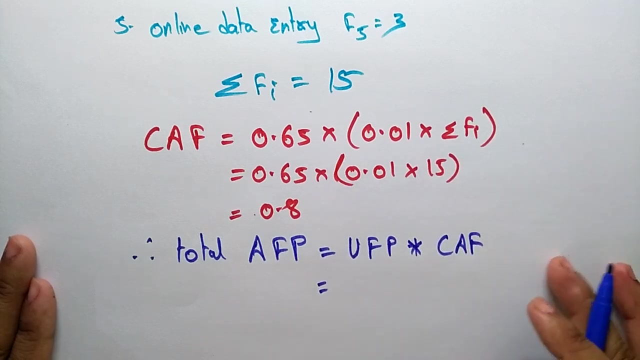 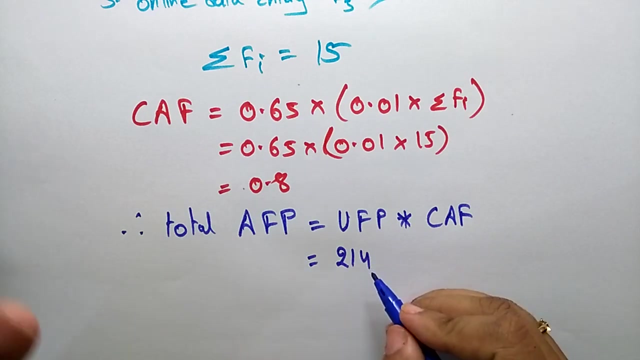 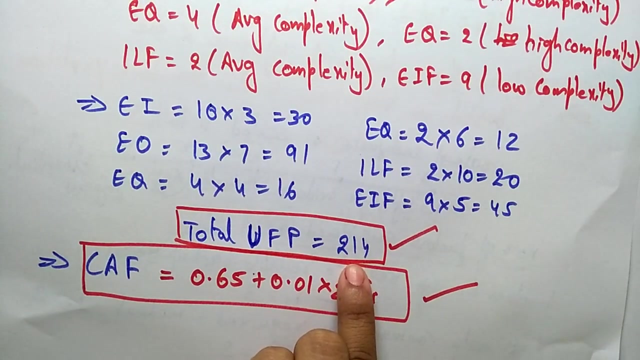 and cf. so the total. therefore total adjustable functional point, afp is equal to unadjustable functional point into caf complexity, adjustable function. so ufp means i'll get 214. i already calculated this. i'll i get 214. so here i calculated. so the total ufp, i get 214.